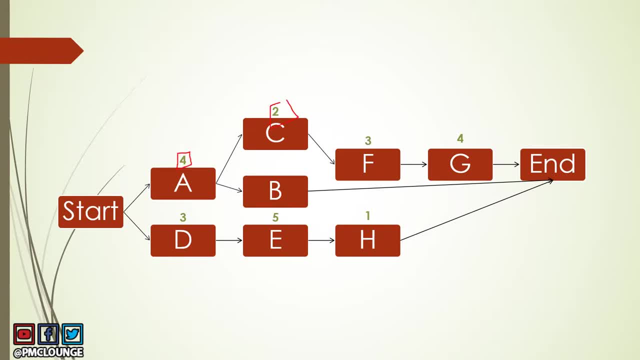 these numbers here right, 4,, 2,, 3, the ones that I'm highlighting right now- these are durations And these A, B, C, all of these are activities. So these numbers were always available in the 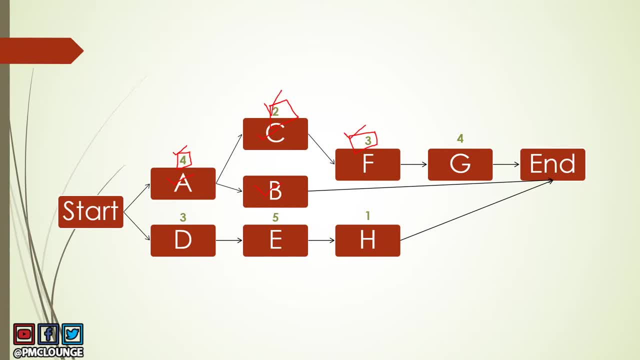 network diagrams. in all the questions, in all the examples that we took, We talked about how to calculate critical path. We then talked about how to calculate early start, early finish, late start, late finish and float, And in all those network diagrams, examples. 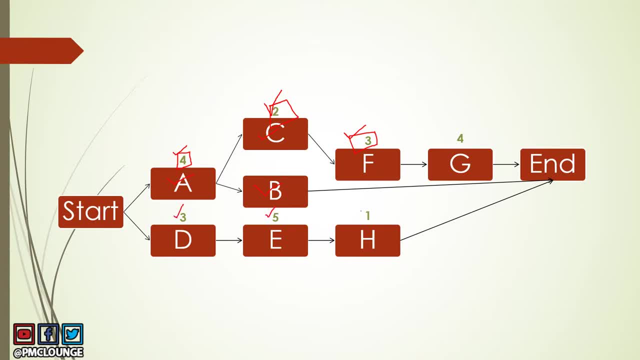 these values of duration was always available, So one of the questions that came in from Twitter was: how do you calculate these durations? All right, This is where we need to look into the basics. This is where we need to look into the PGKA. 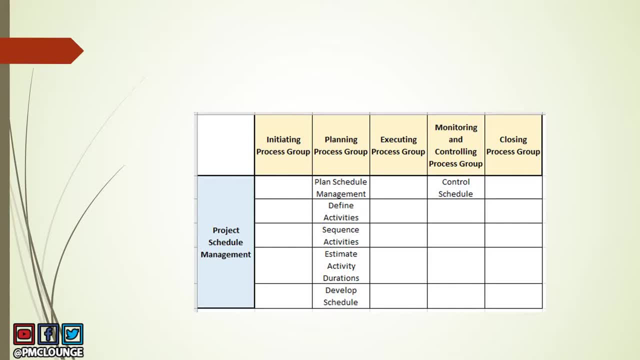 mapping. This is where we need to look into the processes of schedule management knowledge area. So whatever we do related to network diagrams is all about developing a schedule. This is the process we are in when we are looking at the schedule management knowledge area. So we need to. 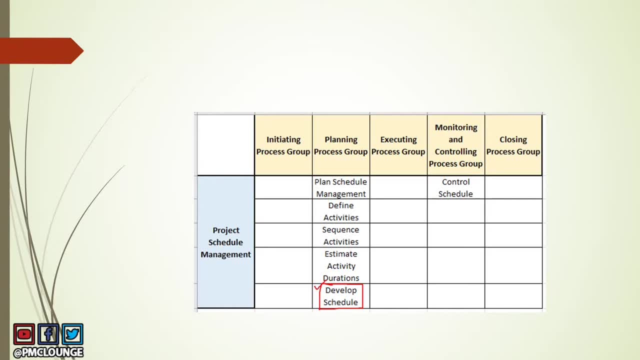 look at network diagrams when we are calculating float, when we are calculating early start, early finish, when we are calculating the critical path, because we are developing the project schedule. So this is where the questions that we are seeing already has durations in them. 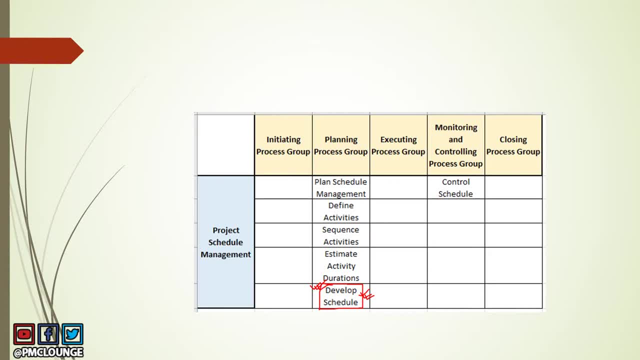 The reason for that is pretty simple. The develop schedule process has inputs from the outputs of its previous process. These are the previous processes. All of these we have already discussed. Second link in the description is going to take you to the playlist of the project schedule management knowledge area. 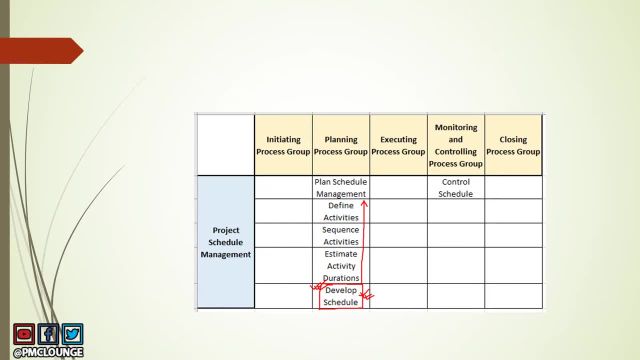 All the videos on schedule management knowledge area, all the topics. So the process just before develop schedule is estimate activity durations. This process, the output of this process, is the duration for the activities And if you remember, if you have been following us,